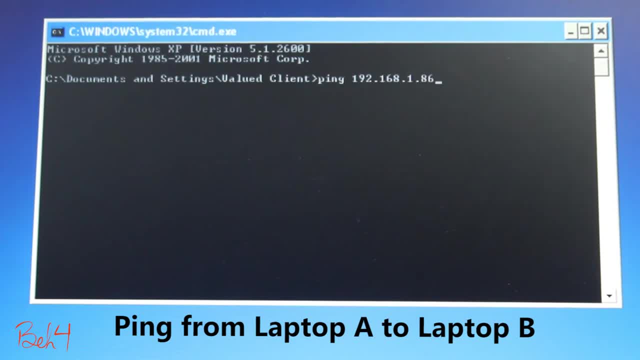 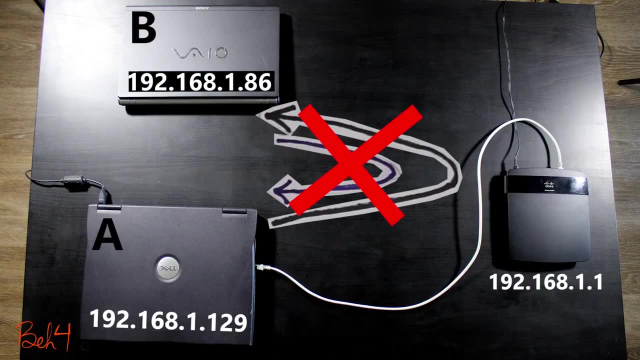 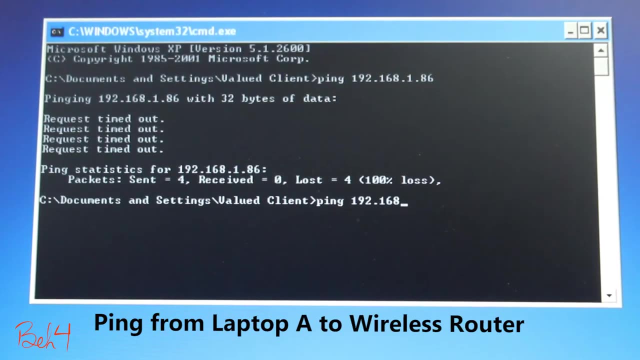 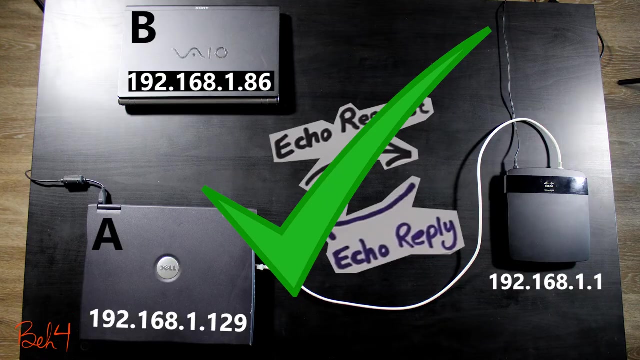 192.168.1.86. No, they're timing out. Let's see if I can ping the wireless router. It's 192.168.1.1. Yeah, that is successful. I'm gonna log into the wireless router to see if the router itself can ping any of the laptops. 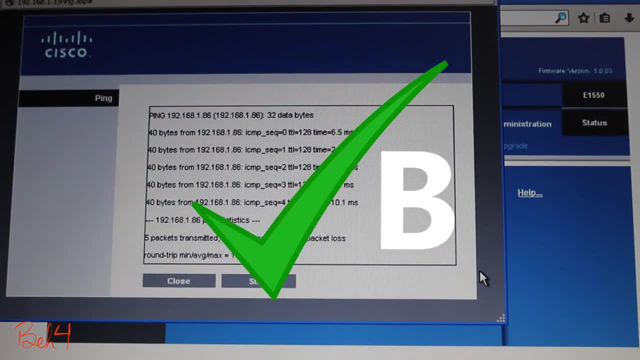 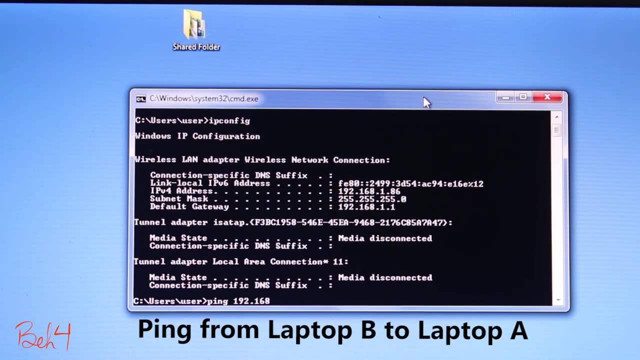 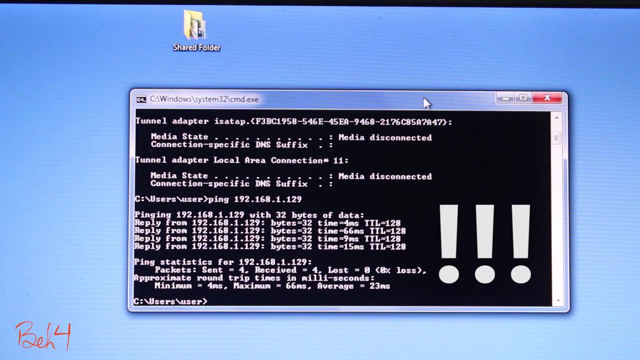 It looks like the router can ping laptop B And also laptop A. Now let's see if Laptop B can ping Laptop A. That would be the opposite direction. What the f**k? That's weird. Everybody's pinging everybody except Laptop A is not. 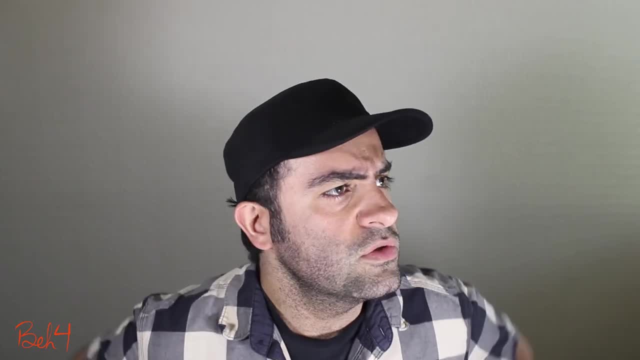 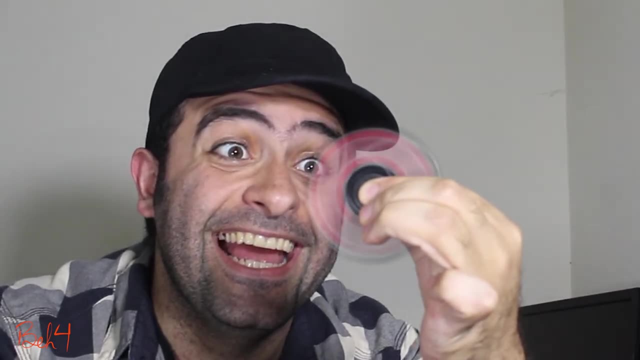 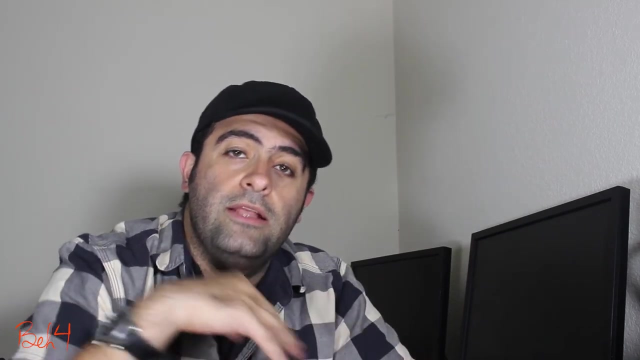 pinging Laptop B. It doesn't make any sense. I need to do something so I can calm down. I have an idea. I'm gonna run a packet captures on Laptop B and run a continuous ping from A to B. Then I'm going to inspect the packets to see if Laptop B 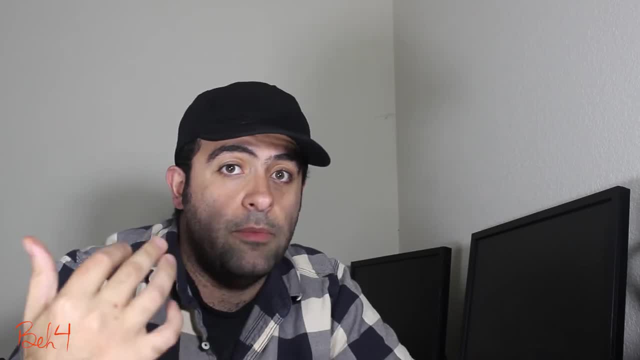 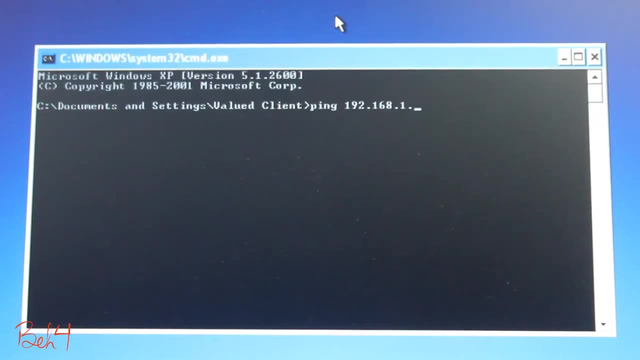 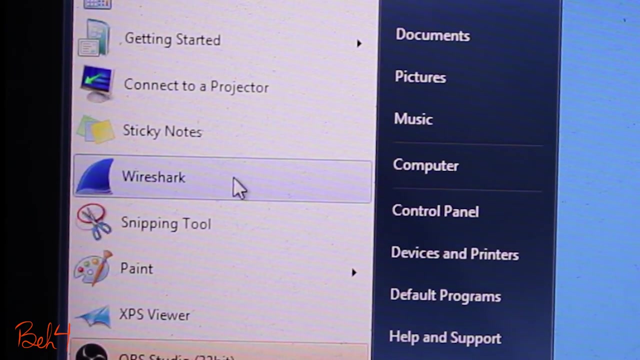 even receives any ICMP echo requests from Laptop A. This will give me a better idea on what device is probably blocking the traffic. Okay, I have the continuous ping running from A to B. I also have installed Wireshark, which is a free packet analyzer software, on Laptop B. When I run the 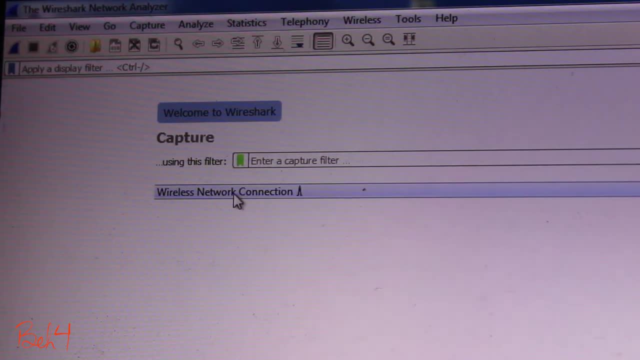 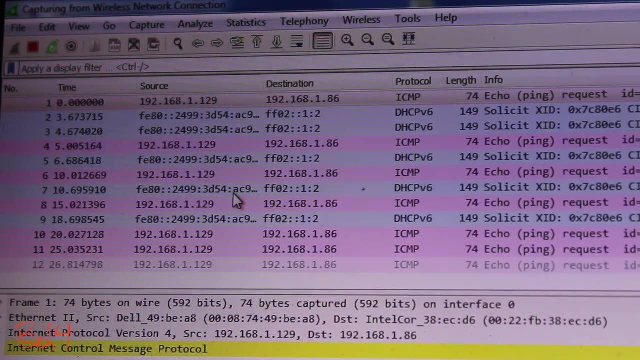 software. I just need to choose the network interface that I want to run the packet. I will run the packet capture and it should start taking the packet capture immediately. I will let it run for 20 to 30 seconds and then stop it, Because there could be all kinds of 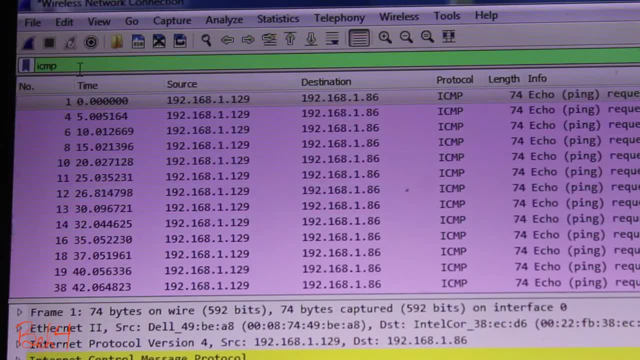 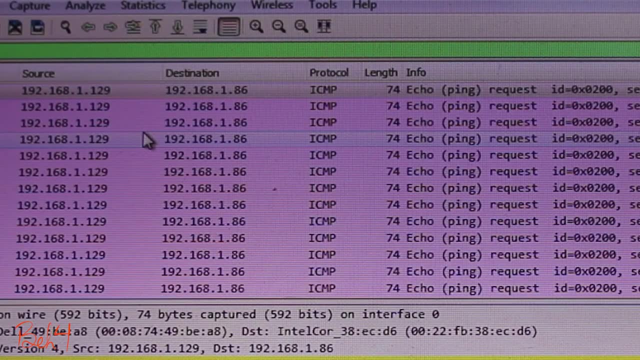 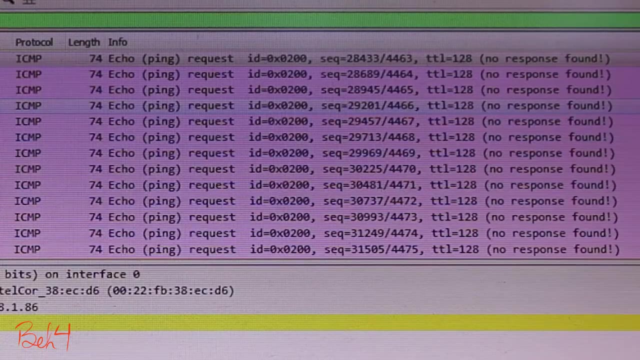 packets here I'm going to filter for ICMP packets only Interesting. So based on this packet capture I can see that Laptop B is receiving ICMP echo requests from A but is not replying with ICMP echo reply. I only see one-way ICMP traffic here. This only tells me that Laptop B is.